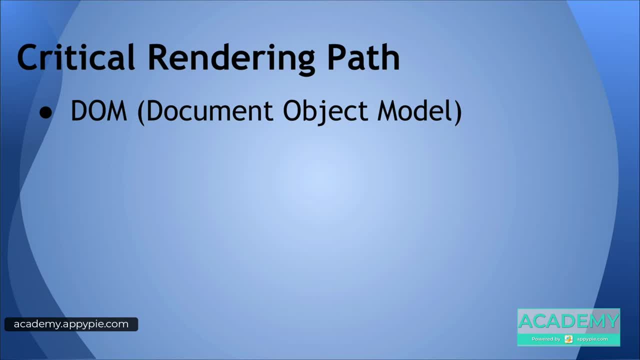 that this means- I'm going to put it in very simple terms for you All- that: the critical rendering path and the DOM. all that this stuff means is that your browser parses the HTML that your page has and it looks for certain things like scripts and images and all the things that are in your page and somehow 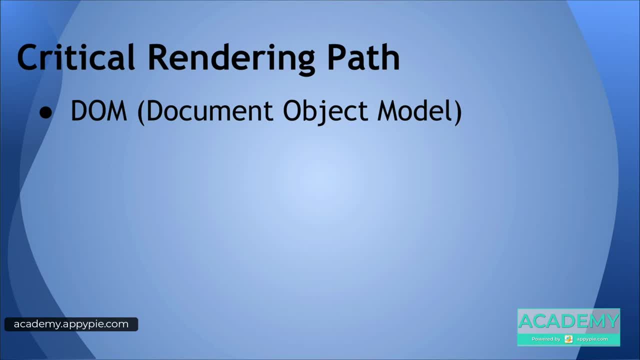 parses it into things that your browser can then use to display the page. That's all it is, And there's a certain path. The critical rendering path is: there's a certain path to doing it And it usually, if you read the HTML from top to bottom, that's really the path, with some examples, Because sometimes the HTML 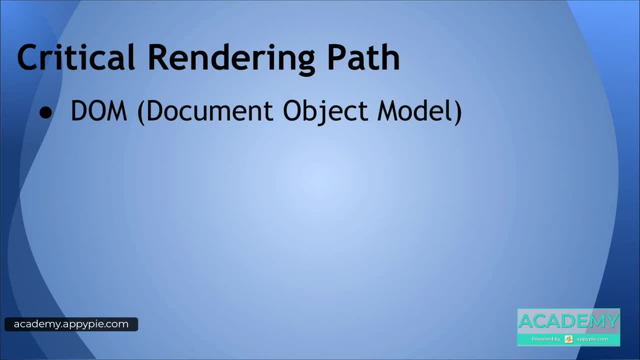 needs to call styling files that have your styling designs you know, or has to call JavaScript files or something like that, And those are. they block the rendering. So CSS is basically cascading the CSS file sheets. This is what gives your page the look and feel, The important thing about them. 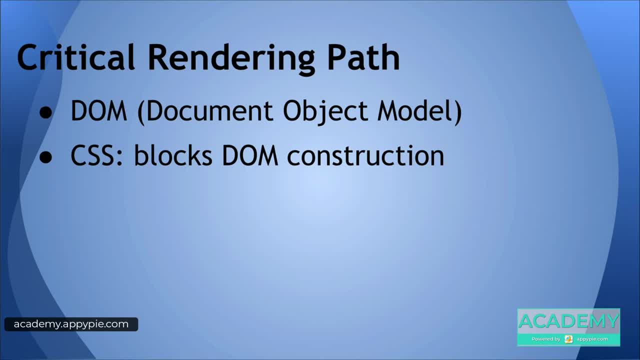 is that CSS files are usually externally referenced, and they are. they block DOM construction. So what that means is your page. literally, when your page encounters a CSS file that it has to externally reference, it literally waits, waits, waits, waits, waits until that CSS file is fetched, And only. 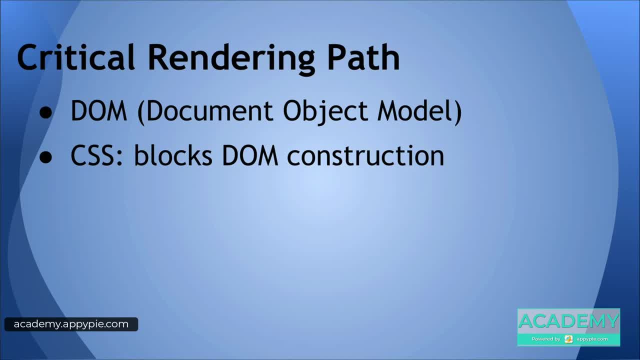 then it can resume displaying. you know, creating the DOM for your page, And only your page, only gets displayed when a DOM is created. The same thing with JavaScript. If your browser encounters a call to a JavaScript file, then it makes that call and waits, waits, waits, waits, waits until. 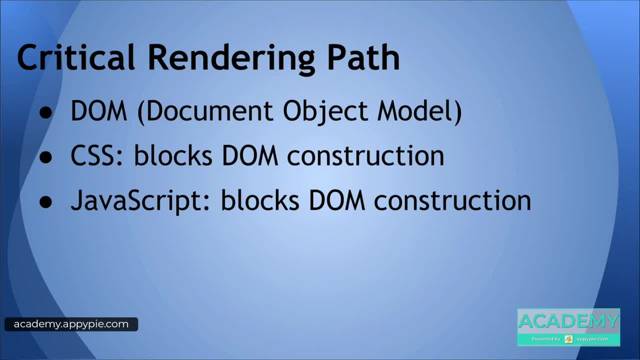 your. you know the JavaScript is fetched and then processed and then your DOM construction can remove. So you see that if you have a lot of CSS files you can do a lot of things. You can do a lot of external CSS calls, JavaScript calls. all these things can slow down your browser If you just 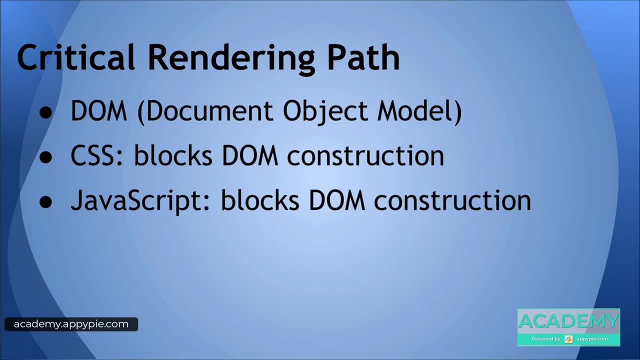 have a few such calls. they're pretty quick, but they can add up. They can add up because they block one another. They have to wait for one to come back to. you know, it's not something that is usually done simultaneously. There are possibilities for this and we're going to talk about later in the 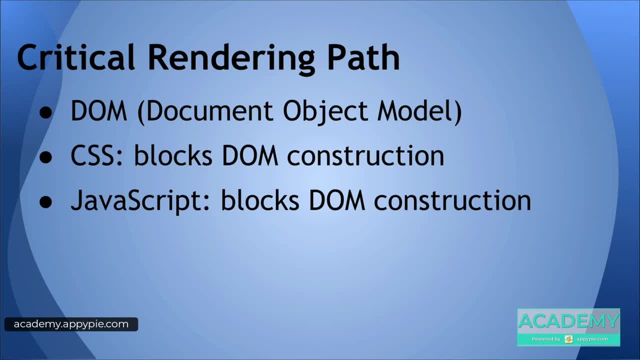 course, but as a default they have to wait for one another, And that's the important point to take away for you is that they slow each other down. They depend on each other, So they can cause a lot of bottlenecks. Additionally, things that slow down your site are large images, So if you 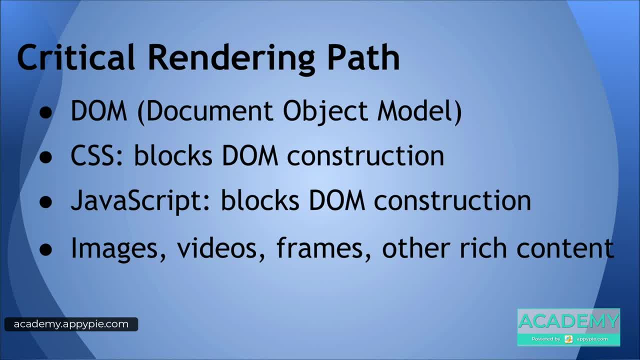 have like beautiful images. it might take a lot of time for your browser to download, So a small image that's compressed might take milliseconds to download, which is which is not something that you would feel when you're as a user. But if it's a beautiful large image, then it might. 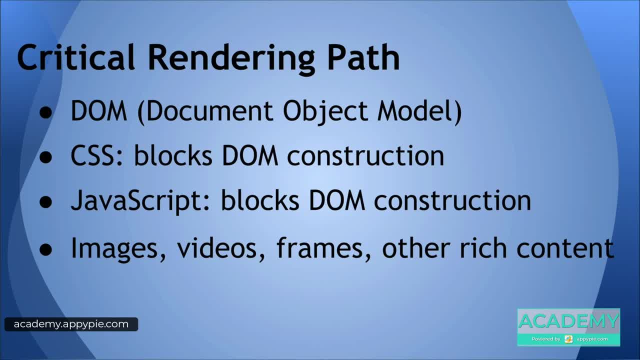 take a few seconds to download because it just takes a lot of space and that might slow down your site. So if you have a lot of these or any kind of rich content, like many you know- high resolution images or videos or frames within your page or other rich content, that really slows down. 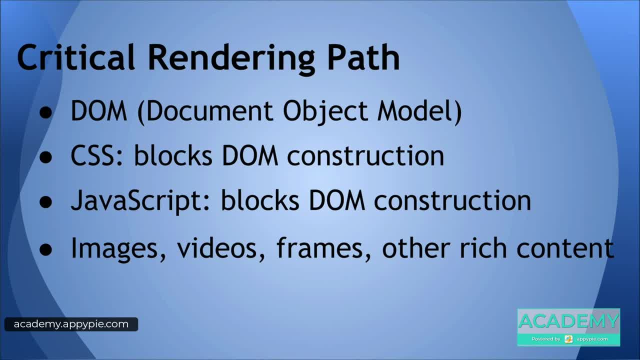 your site. So that's also some something that's pretty easy to examine and identify And you can fix that right away as well. So some of these are very low hanging fruit and we'll get to all the low hanging fruit. So, like within a couple of minutes, we're going to talk about some of the 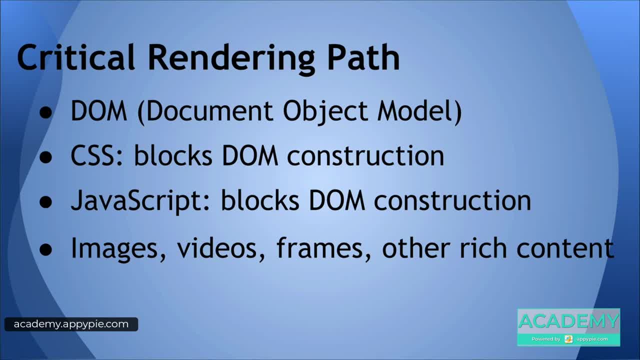 things that you can do to speed up your site. So within a day, let's say within the first 24 hours or within your eight hours of full work on this, which is to say your first day, you can really create a lot of fixes and speed up your site quite a bit, And that's exactly what we're going to end. 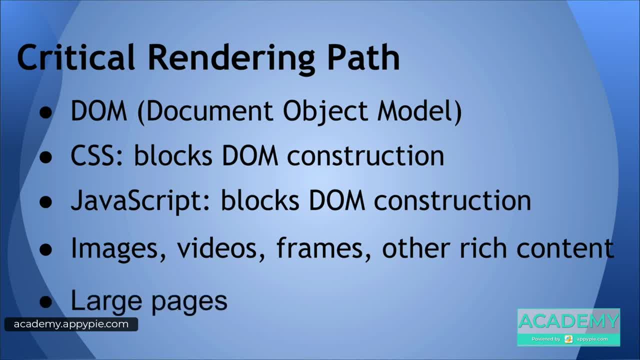 up doing in this course. The last thing I want to bring your attention to is just if you have large pages- all pages these days online. they have images, they have videos, or at least some you know. they have CSS, they have JavaScript or at least some combination of them, So you can get rid. 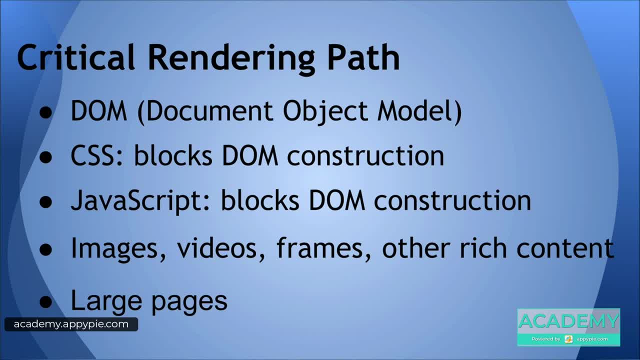 of all these, But what you can do is get rid of many of the unnecessary ones and make sure that a lot of these are totally needed by your page, because sometimes they are causing more slowdown than the benefit that they bring to your users. So a page with a lot of text is not a problem, because text is very